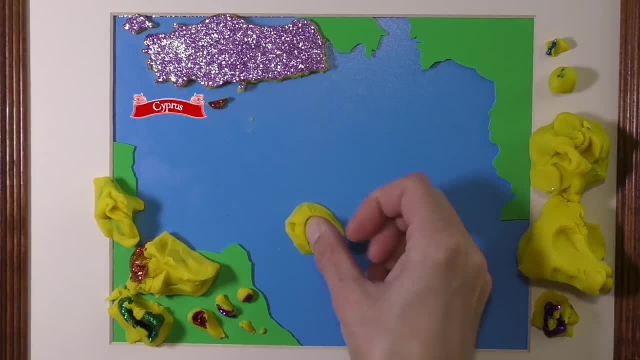 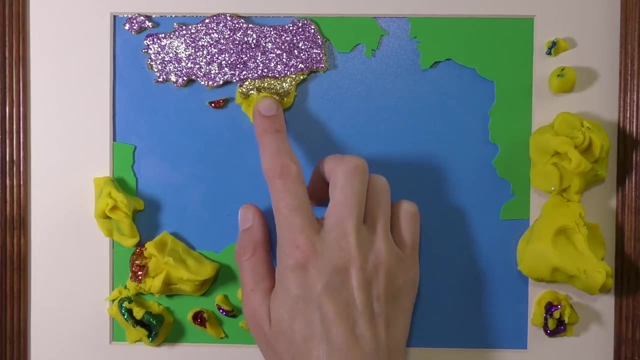 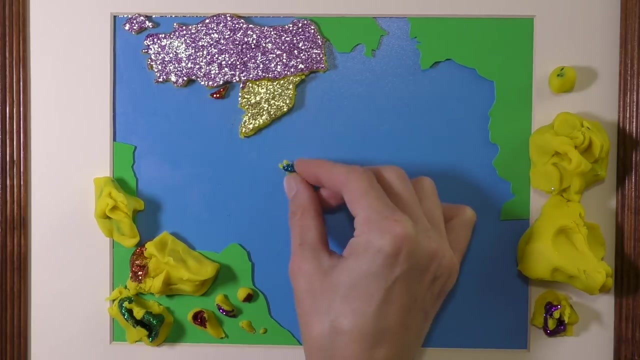 Here's a little one, Oh, that's the island of Cyprus in the Mediterranean. Here's a golden one, South of Turkey: That's gonna be Syria. Another on the Mediterranean, It's Lebanon. What's this? A purple country, That'll be Israel. and 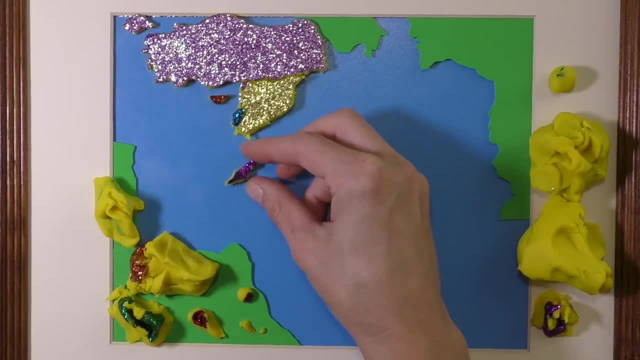 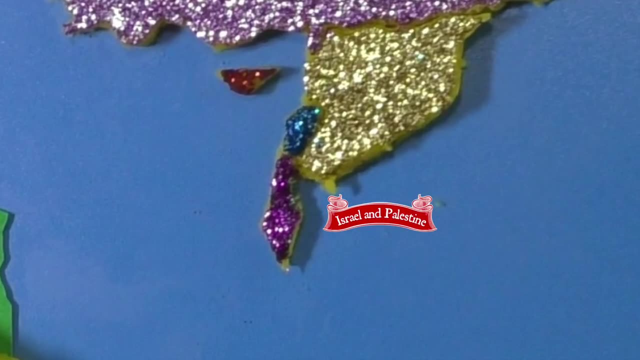 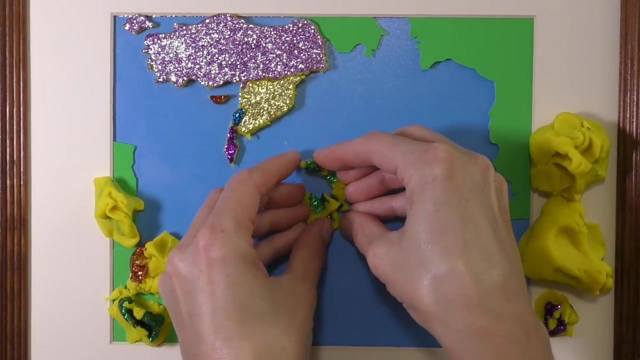 and Palestine. Wait, there's two countries in that one spot. Well, that's complicated, Elise. Let's just say: some of the people there disagree about some things. Let's hope they can work it out. Yeah, I hope so. Whoa, green pieces, Let's stick them together to form Jordan. 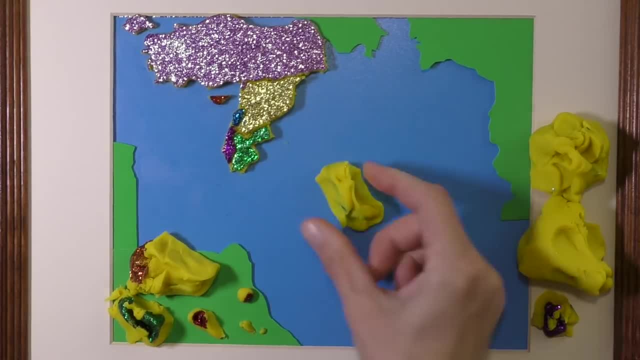 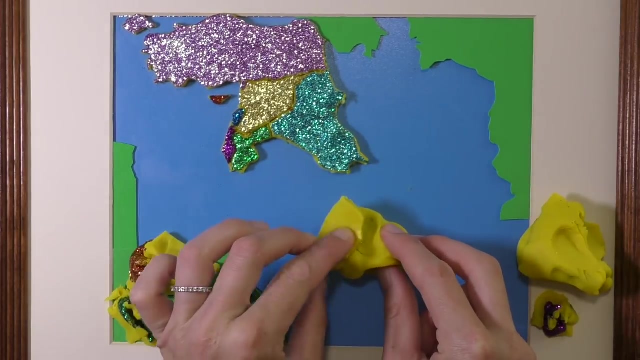 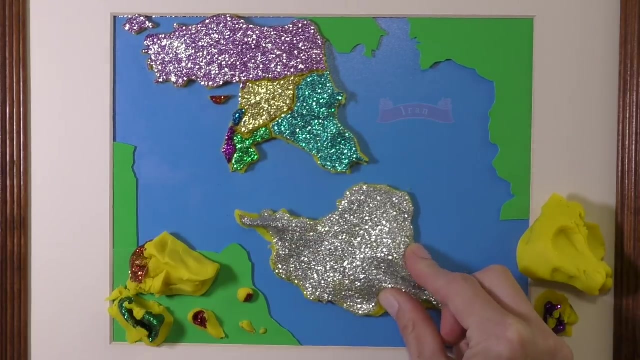 Here's a big one, It's a pretty shade of turquoise. That's Iraq. Another big one in silver To the east of Iraq, That's Iran. Whoa blue pieces pounds on a piece of gold. Hey, here's a big one, It's a pretty shade of turquoise. That's Iraq. 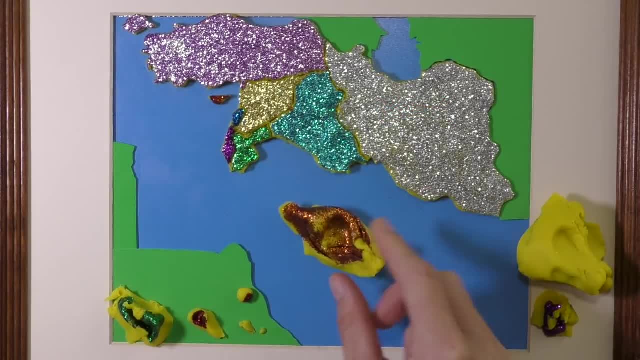 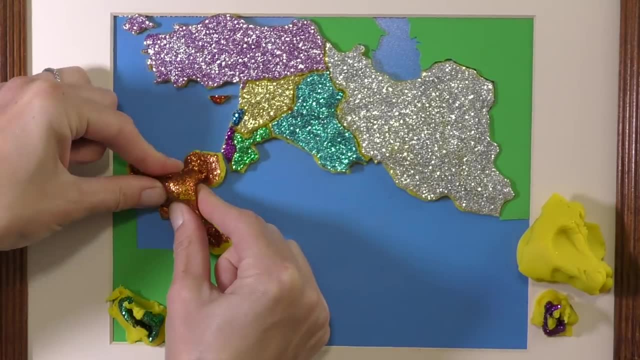 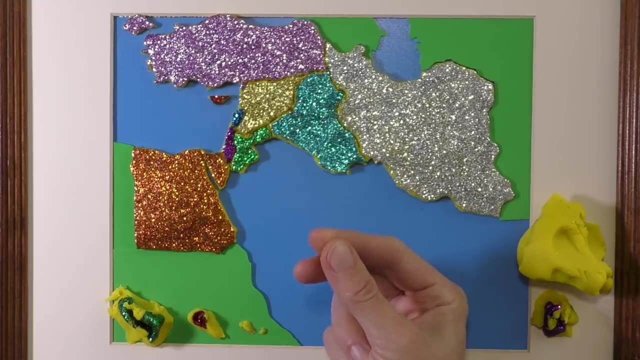 Another big one in silver To the east of Iraq, That's Iran. Hmm, what's this country? I can't tell. It's a beautiful copper color. Oh, over on Africa It has to be Egypt. Now we have Kuwait below Iraq. 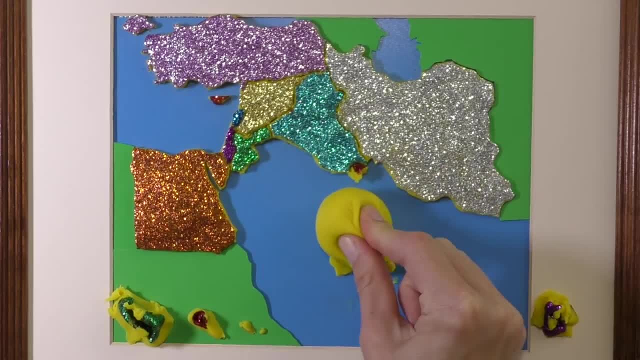 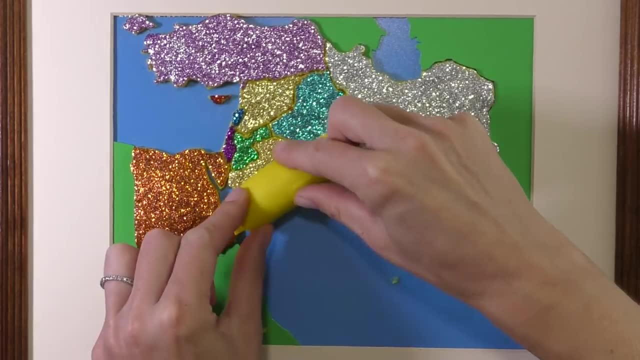 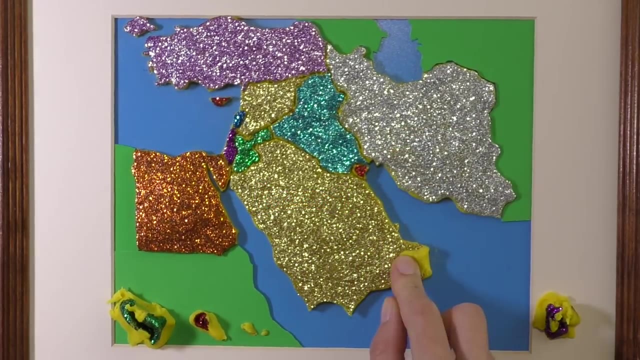 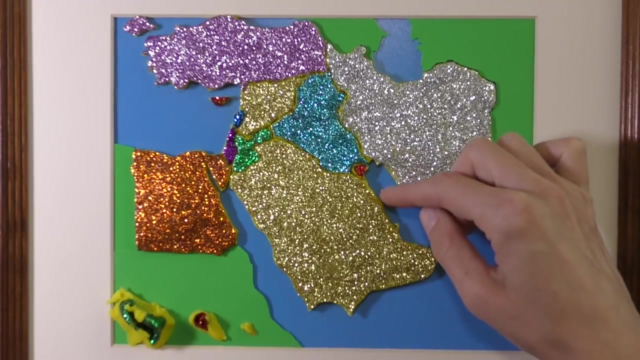 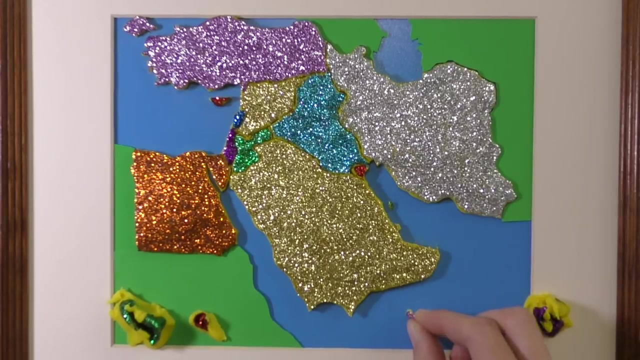 This map is starting to look familiar. Yes, and this next country will really bring it together. Let's unroll Saudi Arabia, But there's more on the peninsula: There's Bahrain, And there's Qatar And the UAE. Here's another purple place.